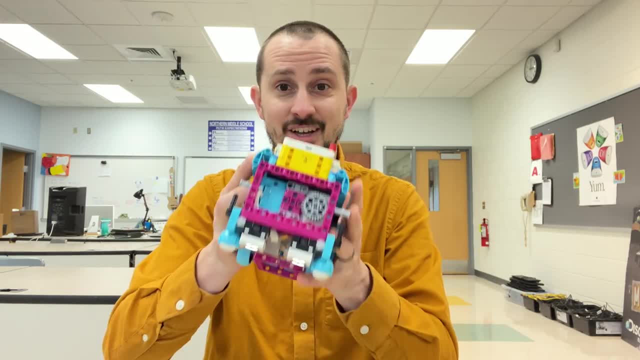 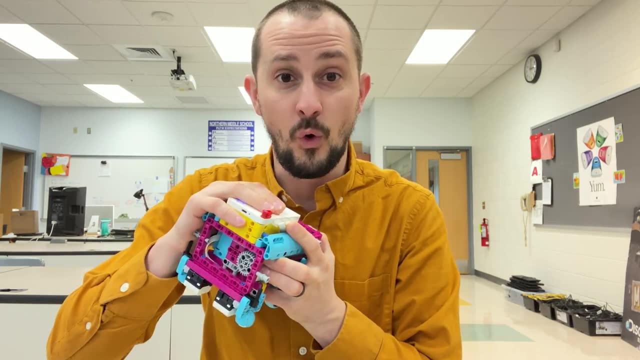 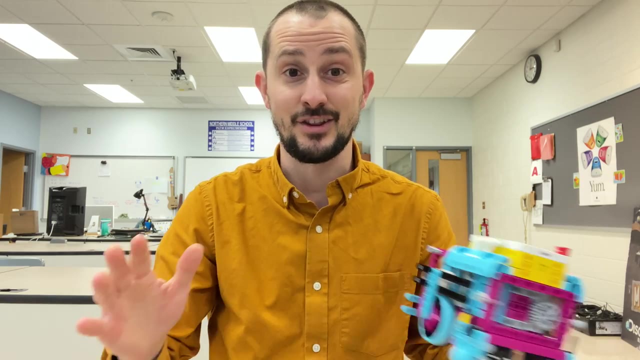 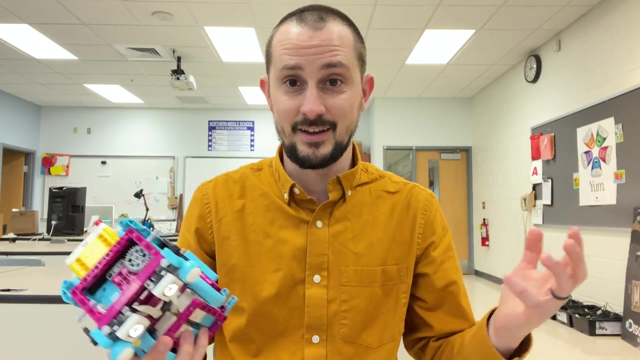 Okay, we are going to. we're going to talk about how to turn and move a Spike Prime or EV3 robot in the new programming environment that LEGO Education has given us. I think the programming environment is awesome. It looks like scratch programming. It feels like scratch programming. It's awesome. I love scratch programming. The drag and drop blocks- good job. 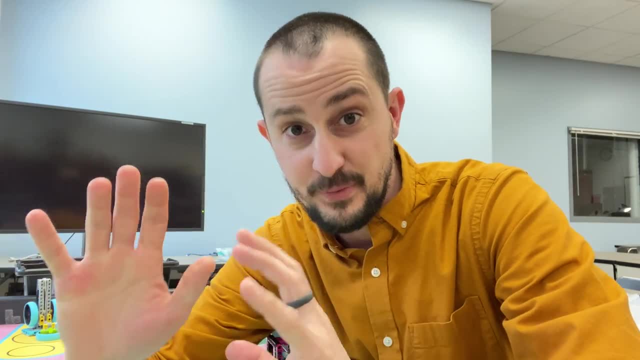 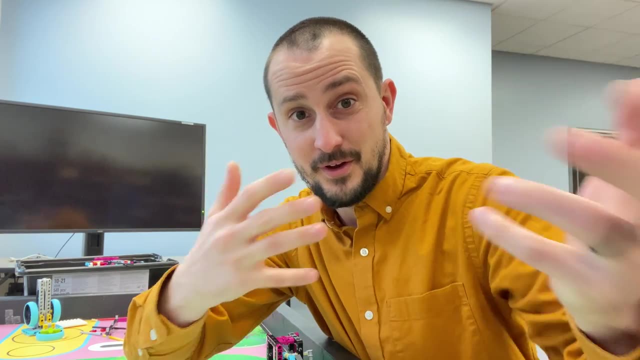 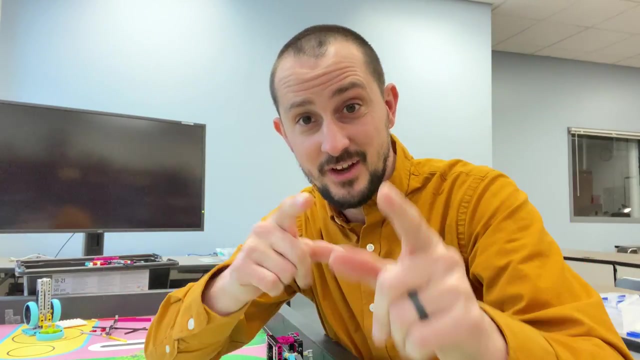 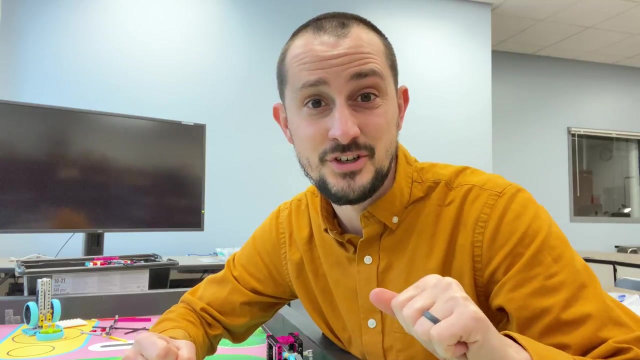 Good job, LEGO Good job. Before I begin, I want to give a shout out to a team that I've met through video: Almost Heaven Robotics out of Parkersburg, West Virginia, which isn't too far away from me. I hear you guys are doing some awesome things. I talked with your coach. She said that you are doing fabulous. 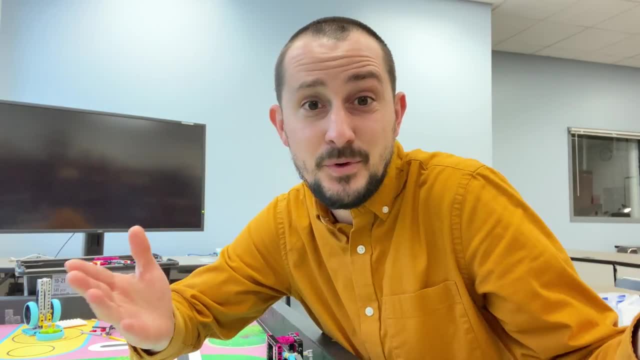 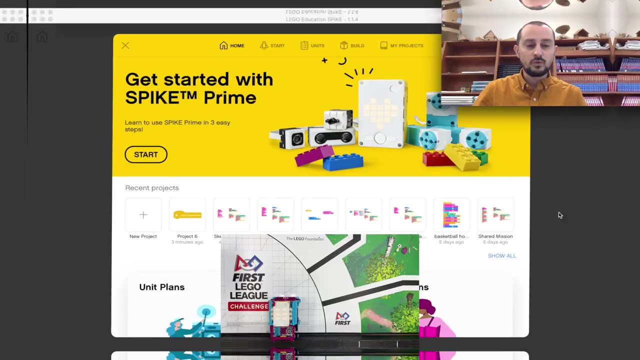 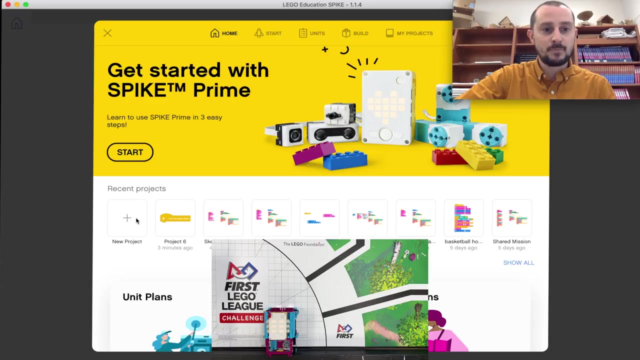 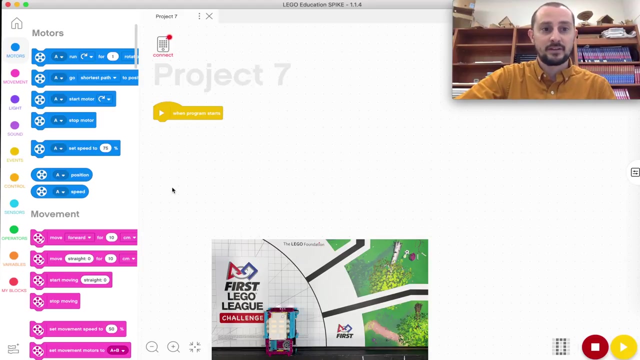 Good luck And maybe, maybe we'll get to hang out. So I am in the Spike Prime programming environment. I'm just going to launch a new program And I'm going to go ahead and connect my brick. That's the first step. So I'm going to click my little brick icon here, my Spike Prime brick. 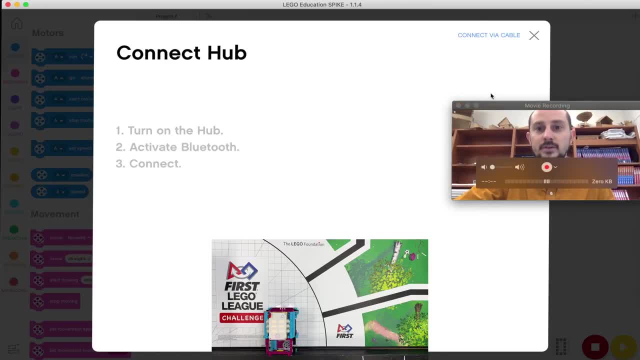 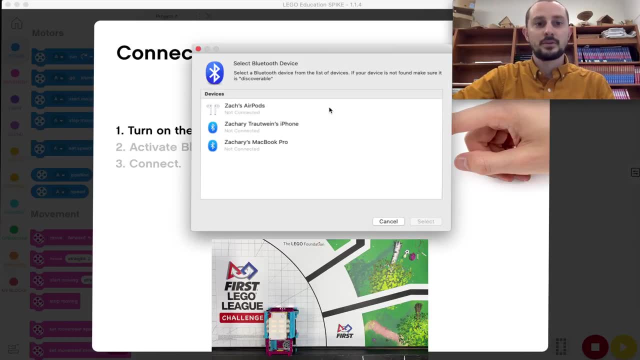 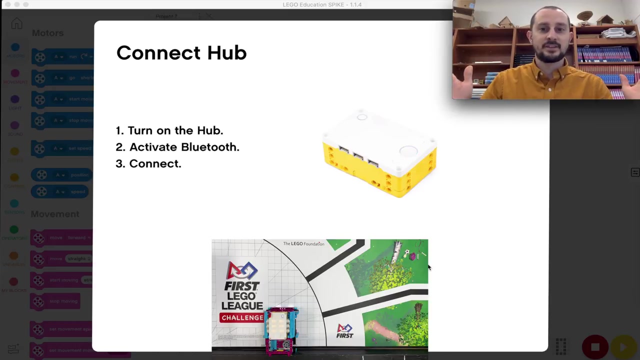 And I am going to select connect via Bluetooth And then press the Bluetooth button on my brick. It'll beep. Bluetooth will come up on my computer And so will the Spike Prime. I'm going to select it. We get the connection sound and we are good to go. 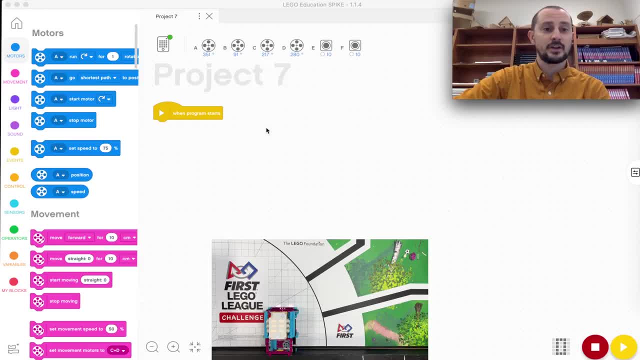 So the program window comes back and we see our project and we see our programming area and all of our bricks and blocks on the left side, Just really quickly. today we're going to be talking about the blue and pink movement blocks and how to program our robot to do some basic moving. 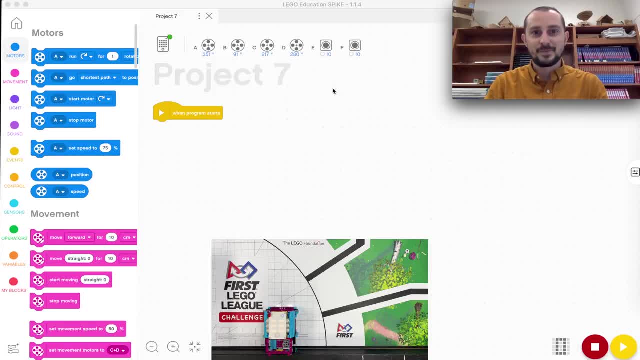 I'm just here to get you started. I'm not here to program full first Lego League missions or classroom missions for you. So before I do anything else, I want to put the brick into streaming mode. I'm going to click down here on the little zero tiles and I'm going to put the brick into streaming mode. 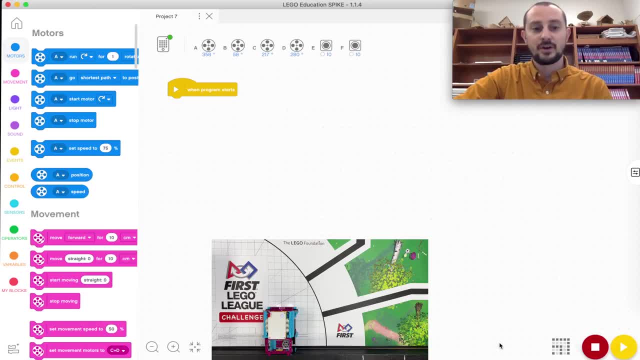 You'll see the little brick flash and the icon change and we are ready to start programming. Now I want to encourage you. I want to encourage you to start programming. I want to encourage you to start programming. If you're going to move more than one motor at a time, I would encourage you to use the pink moving blocks. movement blocks. 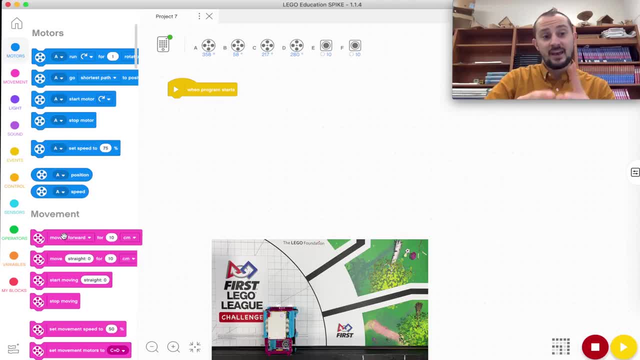 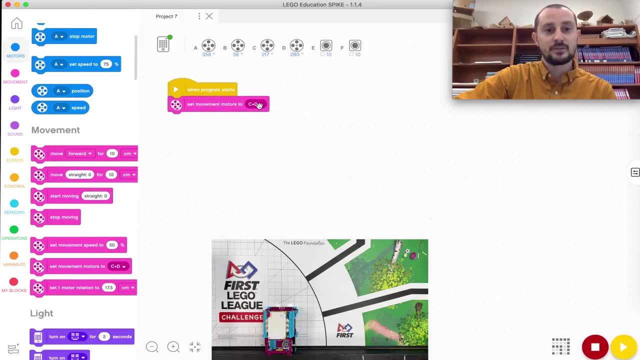 So what this does is it says at the very, very beginning of our program: we can set the movement motors. So anytime we use a pink block, we're going to set our movement motors to A and B or whatever they are on your robot. 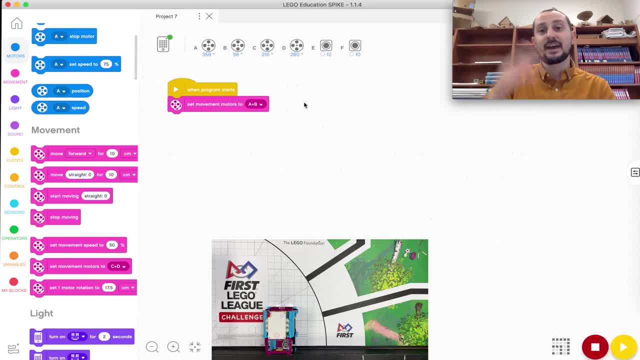 It could be B1.. It could be B2.. It could be A and C, or E and F, or A and F, whatever It doesn't matter. So whatever they are, you can set them as that minor A and B. So then I can just say: move forward. four: 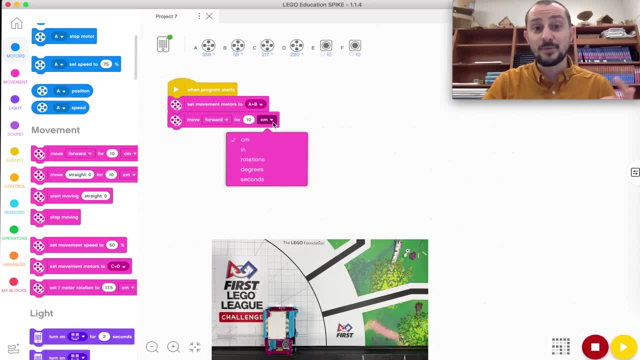 We'll kick it back to the traditional EV3 programming where we don't have necessarily centimeters and inches, but we do have rotations, degrees and seconds. I'm going to say move for 1.5 rotations. And now, if I run this program, the robot will move forward for 1.5 rotations. 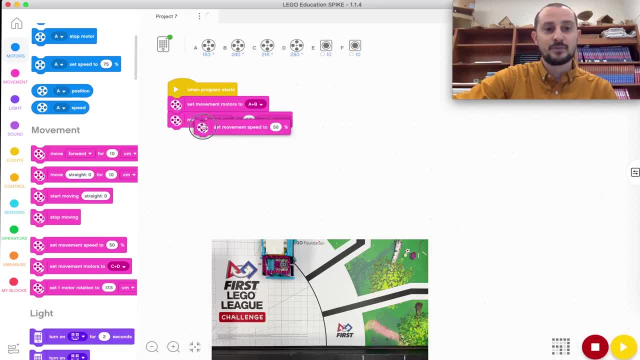 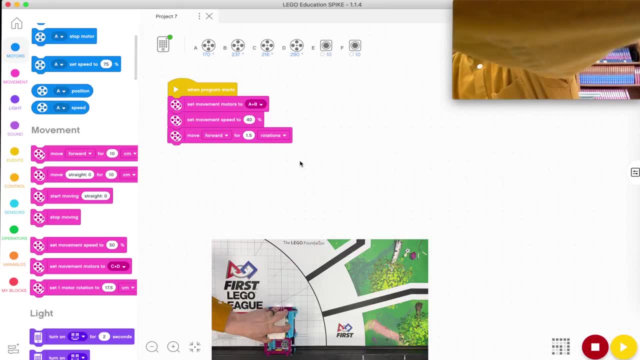 I can change the speed of that by saying set movement speed to. I don't know. I'm going to do 40.. 40 is a good speed. 40 is a good speed for this robot. I'm going to do 40.. 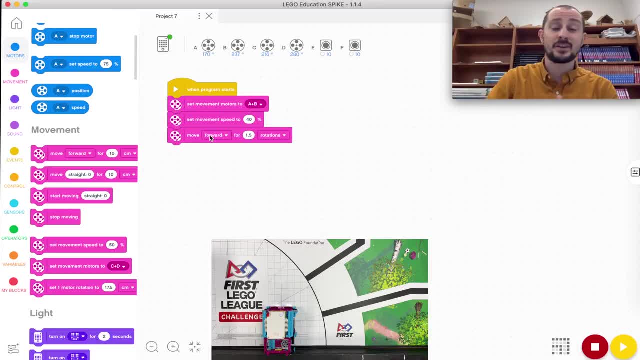 I'm going to use whatever speed is good for your robot, because you might not have the same robot as I do. All right, If you do, awesome, If you don't, maybe you want to check it out. Build video will be linked down below in the description. 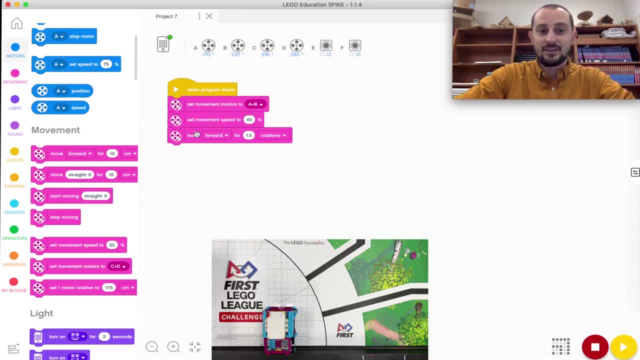 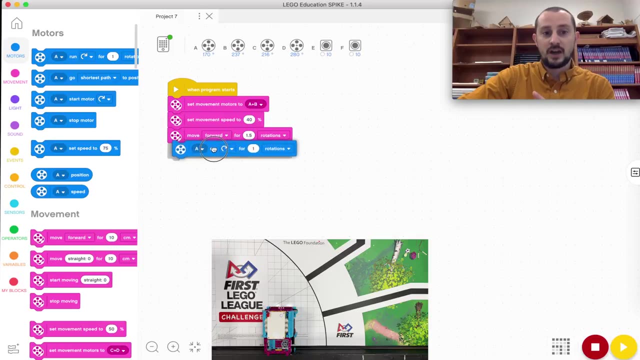 So now I can turn if I want to. There's a couple different ways to turn Now. one of the ways is to just use a blue block and say I want A to turn for B. Let's say I want a 90-degree turn for a certain amount of rotations and I can run this by trial and error to see I want a 90-degree turn. 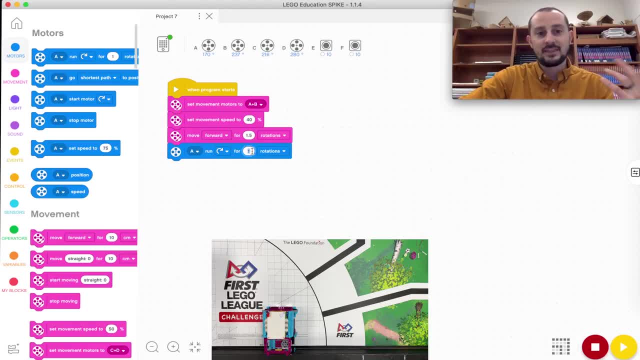 Let's just say I want a 90-degree turn. I can say, okay, well, I think a 90-degree turn is going to be- I don't know- 0.75 rotations, And I can run this and see what happens. 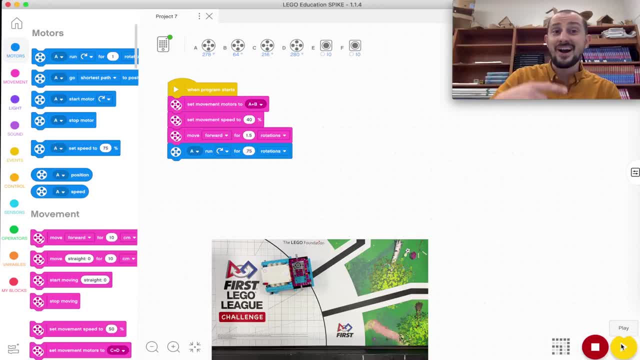 I was actually really close, Okay, But I wanted to turn the other way. All right. So if I want to turn the other way, I'm going to switch. I'm going to switch the direction of motor A and I'm actually going to tell motor A to slow down, because I thought that turn was a little fast. 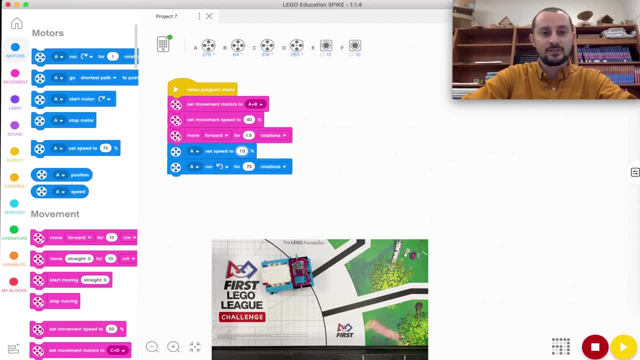 So tell motor A. I'm going to bring a block out and say motor A, slow down to maybe 20.. Programming tip- This is key: Always turn slower than you. drive forward and backward. If you're turning your robot, always drive slower. 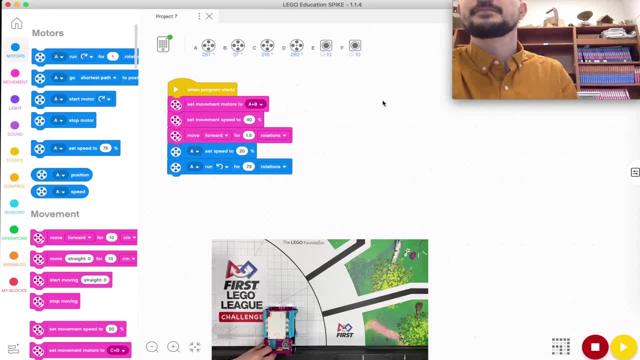 All right. So now, if I reset the robot, let's see what happens. I'm going to put this. it was a little much, but I'm going to keep it as it is. We'll run the program. Oh, that was almost perfect. 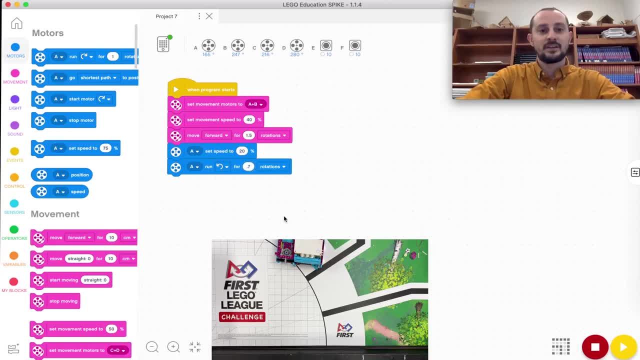 So I think maybe 0.7 on the turn will work. Reset the robot and run this one more time. Maybe we'll get closer to 90 degrees, Maybe not. Put it back to 0.75.. And that's how you decide how far you're going to turn. 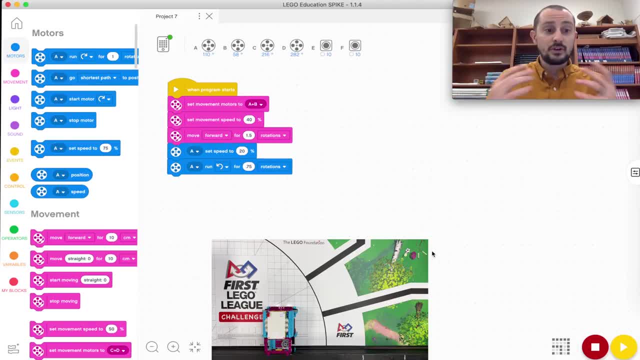 Now you could also turn the other way by selecting another motor. I could say: I want B to turn as well and probably switch direction. That would turn the other way. There we go, 90 degree, turn the other way. And then I could continue on how I wanted my robot to perform in FIRST LEGO League or in a classroom setting. 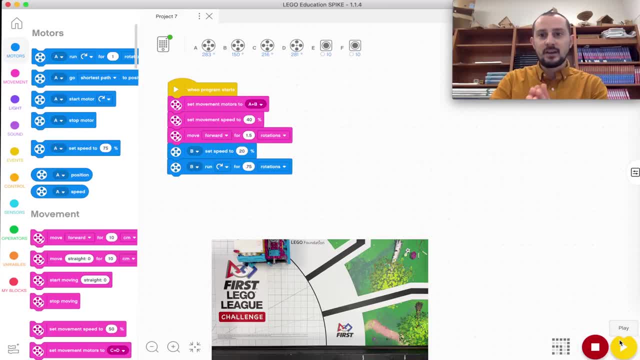 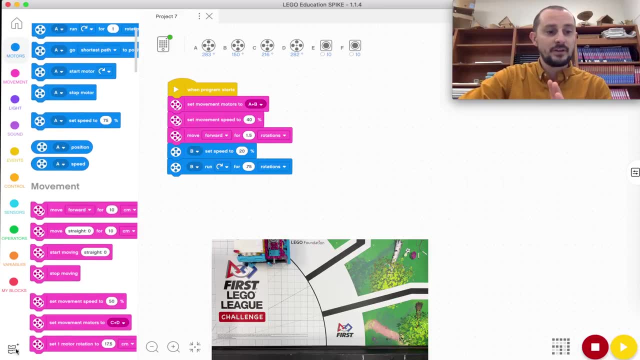 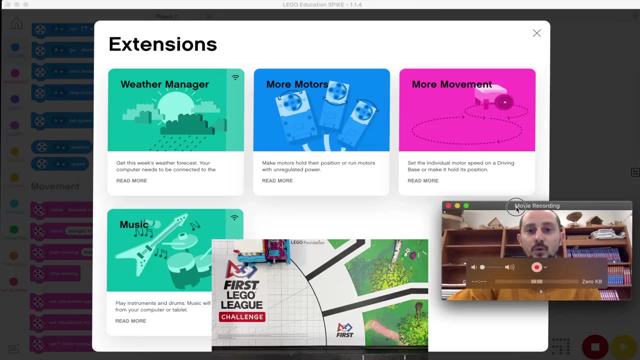 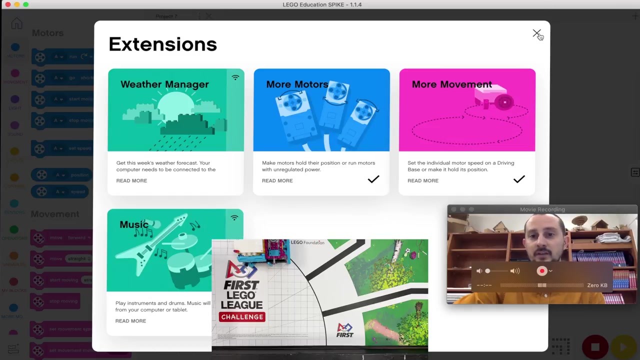 Now I want to show you really, really quickly, there's more movement blocks that you can use. So if we click on the plus bricks icon down here, there are more movement blocks and more motors. I'm going to go ahead and add both of those to my toolbox. 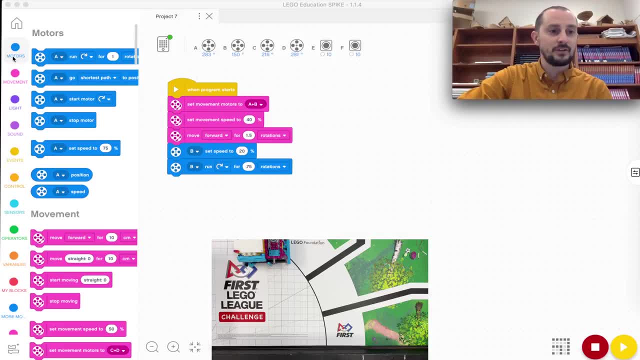 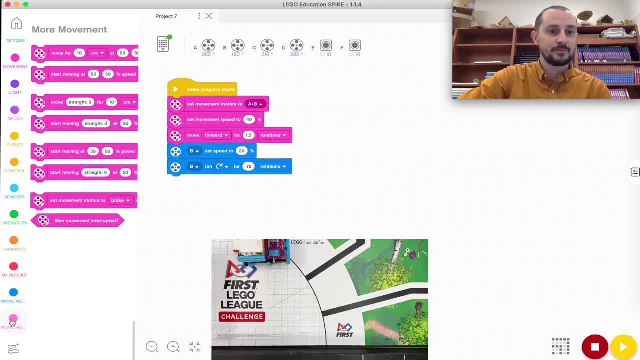 I call this my toolbox over here. Now, if you notice all the way down here, there's more movement and more motors, So you can kind of condense blocks like this. I'm going to write the same thing over here. I'm going to right-click and duplicate this and put it over here. 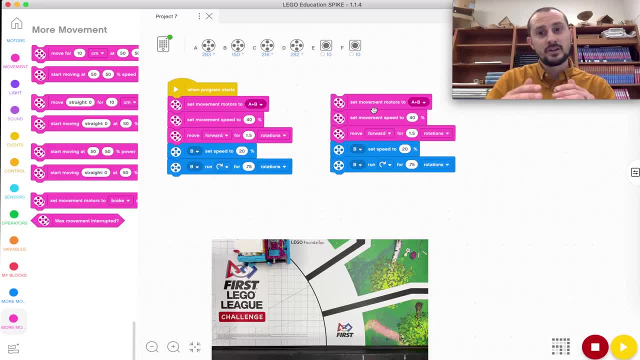 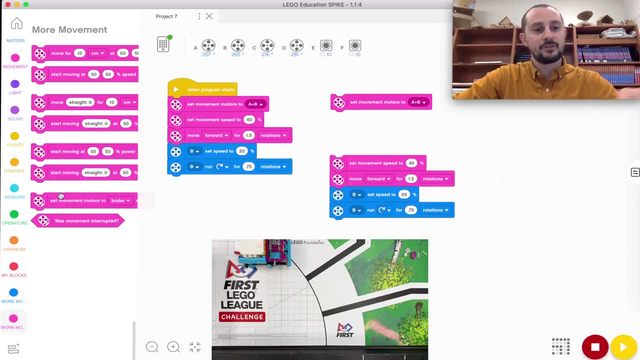 And I'm going to write the same exact code, just condensed a little bit more, less blocks. So I'm going to say I want to move straight. That's the same thing as forward for 1.5 rotations. 1.5 rotations at speed 40.. 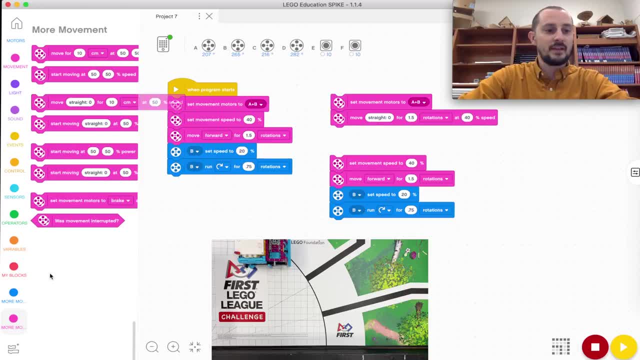 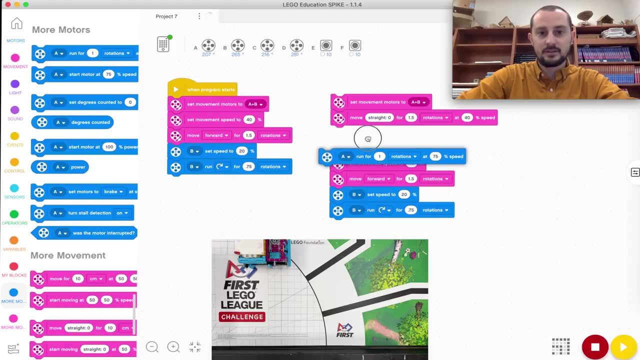 So that takes these two blocks and puts them into one, And then I'm going to come to the movement blocks And I'm going to say I want to run motor. I'm going to go back to the whole motor A thing. Motor A for one rotation at 20% speed. 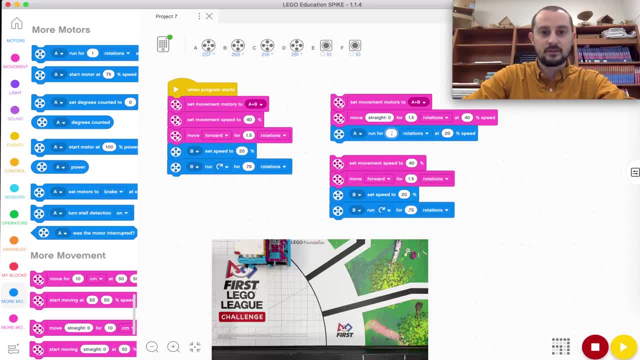 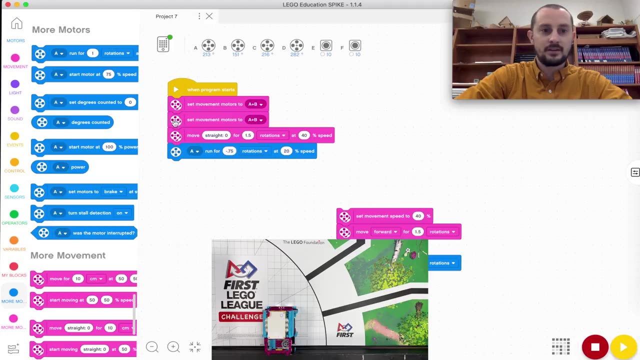 And actually this is 0.75. And I believe I had to switch the direction. Let me get rid of that and put this on. I don't need to set motor A again, So it should do the same exact thing. It should go 1.5 rotations and then turn to the right. 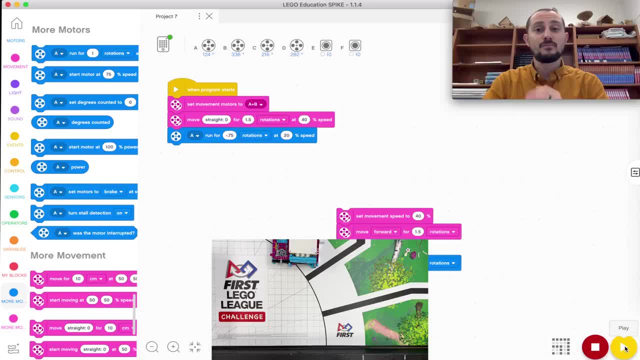 Yep, perfect, And that's some basic moving for your motor Robot. Now, obviously, if you want to go backwards, you can do speeds of or rotations of negative rotations. So if I wanted to go backwards, so say after that I did want to go backwards. 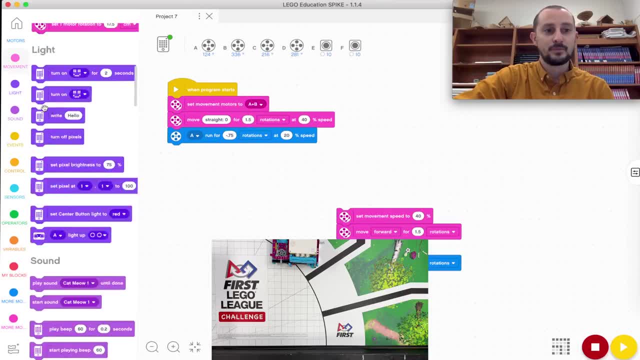 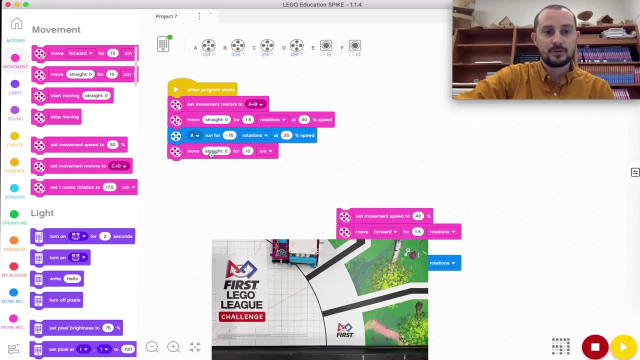 I could say: move in, the movement blocks, the regular movement blocks, There's a move backwards. Or I could move: Move straight for negative rotations, So move straight for negative rotations. Reset the robot And run this And then it moves backwards for negative. 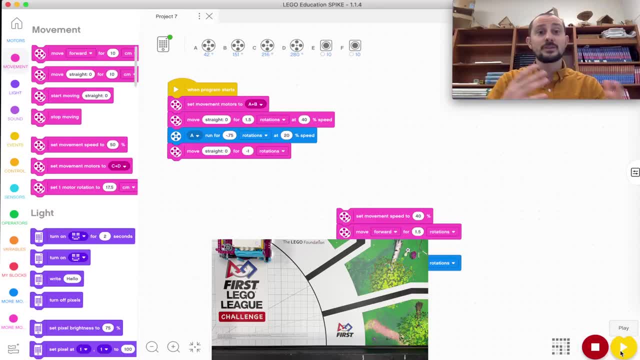 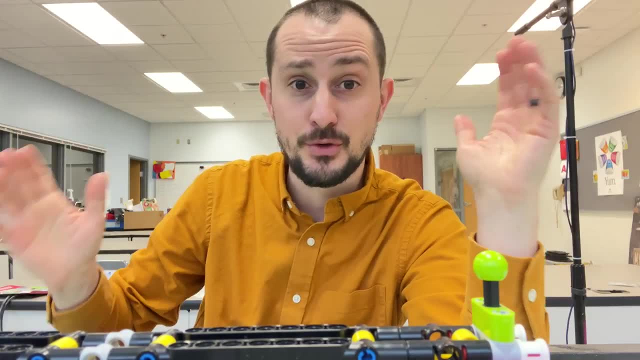 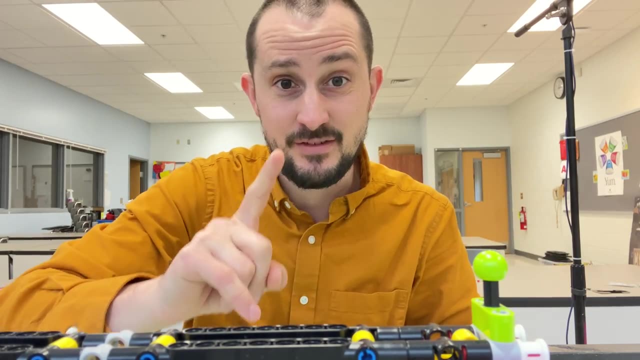 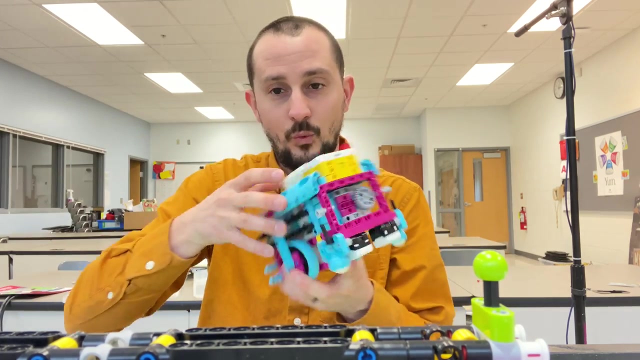 It actually moves negative one rotations. So that's how you can manipulate your robot: by moving it very, very easily. That's it. That's some super basic moving. Now I do have one massive issue with turning Right. So what if something gets in the way? 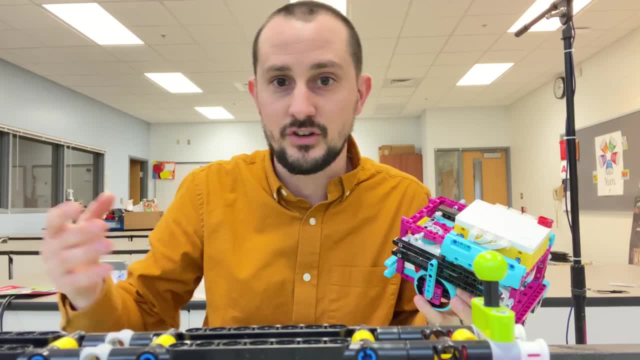 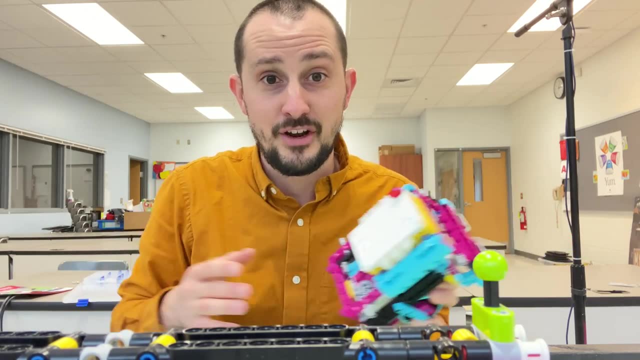 What if your wheel slips? Or what if your wheel is dirty? There's a way to always turn whatever degrees you want to turn or whatever amount you want to turn. That's using The gyro. I'm going to talk about that in the next video. 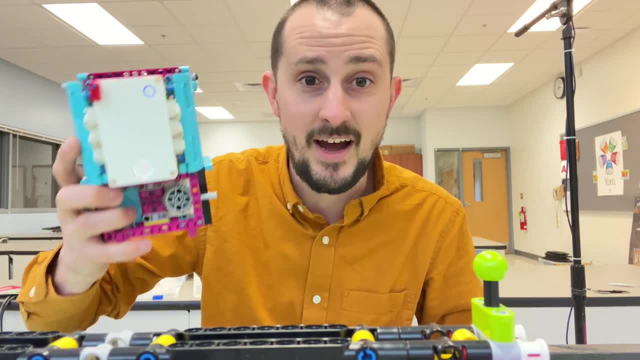 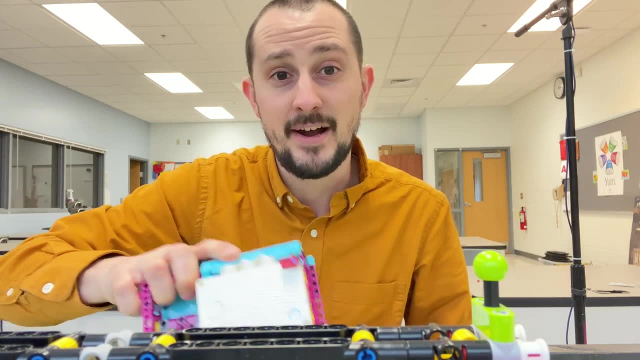 So, whether you have a spike prime or a gyro on your EV3 robot, the next video you're going to want to watch to learn how to program your robot to turn by the gyro- And always make sure you turn the amount of degrees you want to.